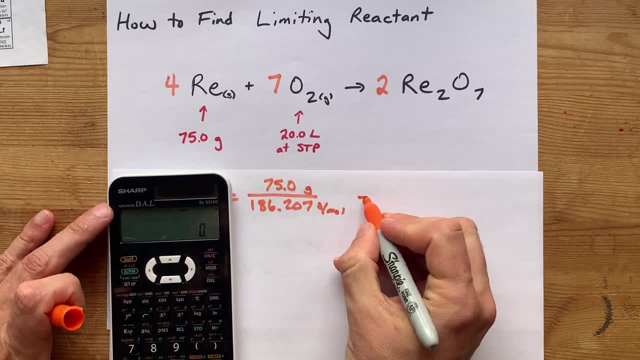 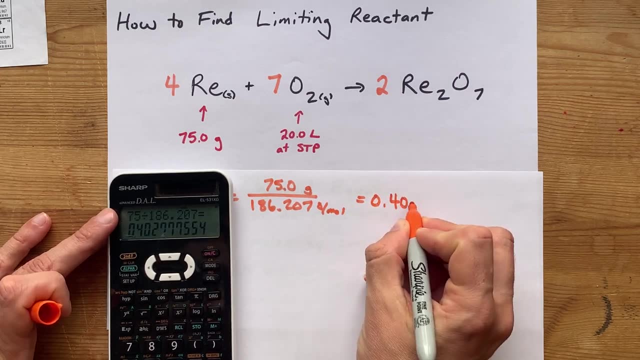 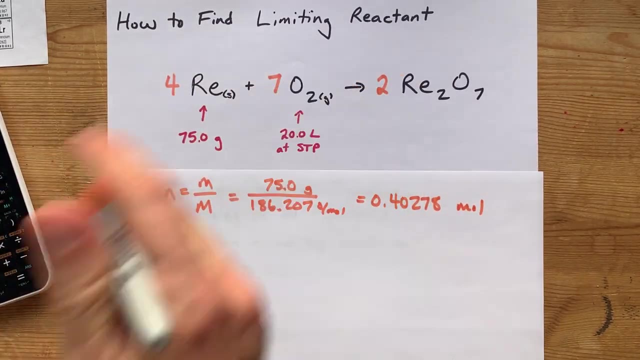 that number of grams per mole, you get the number of moles of rhenium you have. That's 75 divided by 186.207, 0.40278 moles of rhenium. Now oxygen. here is a gas, If you know how to convert. 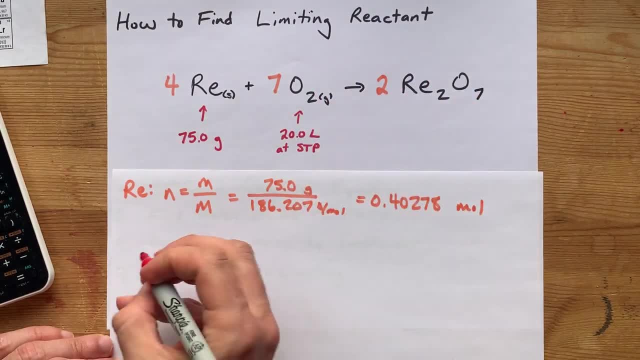 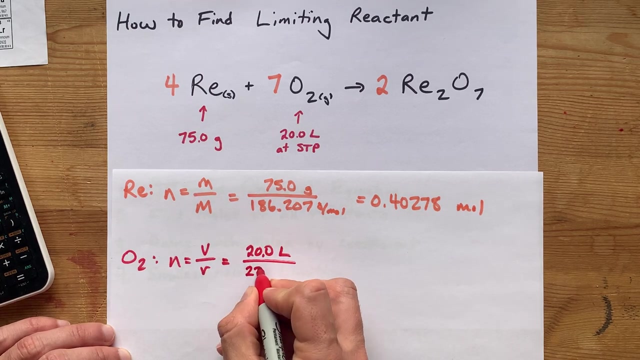 well, liters directly to moles from STP, then you can do that. I happen to You. take the volume and divide it by the molar volume at STP. In our case we have 20 liters and we're going to divide that by 22.4 liters per mole. If you don't know what molar volume is, 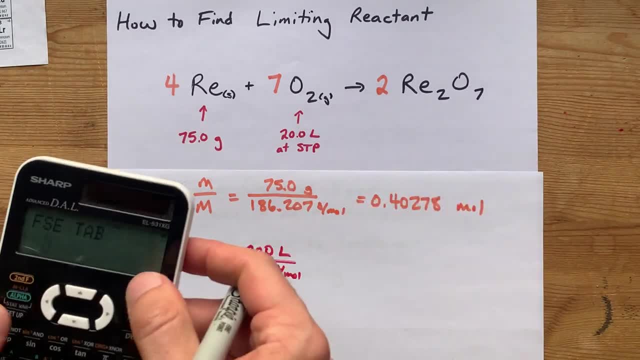 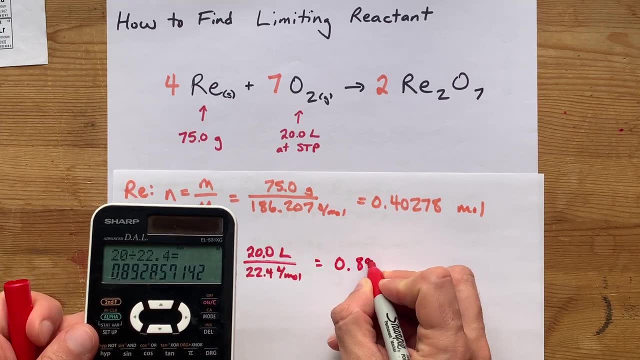 you could always use. PV equals nRT, et cetera. 20 divided by 22.4.. Again, don't worry if you're not familiar with this method of calculating moles. It's just an example. I use to mix. 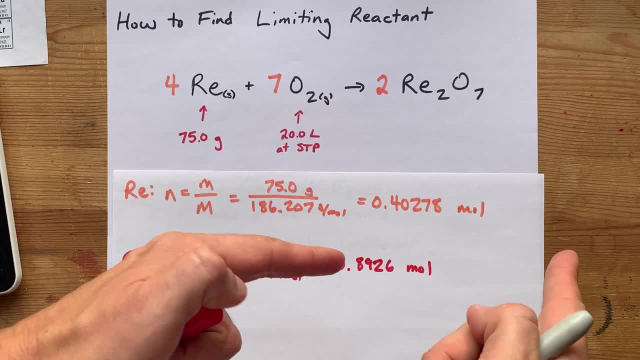 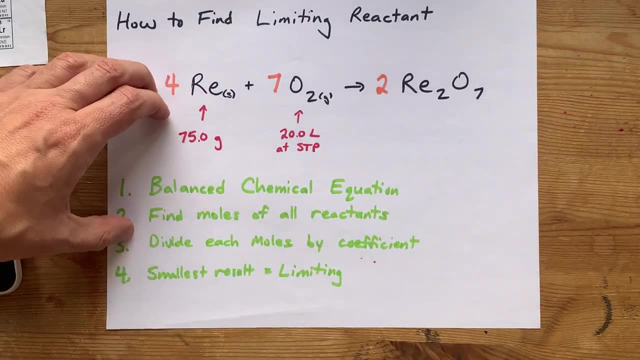 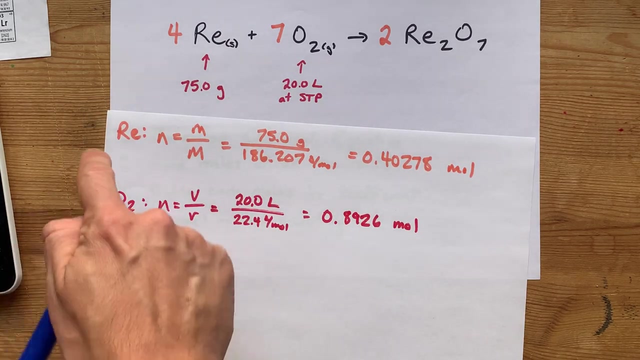 things up. Your job is to convert the amounts you're given into moles. 90% of the questions are going to be grams to mole with this formula. Next step three: divide each of those numbers of moles by the coefficient from the balanced chemical equation. So rhenium will get divided by 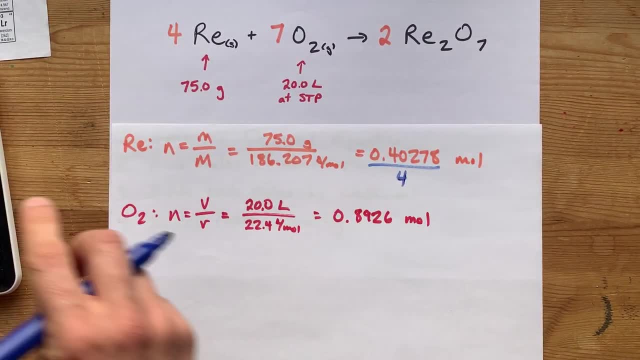 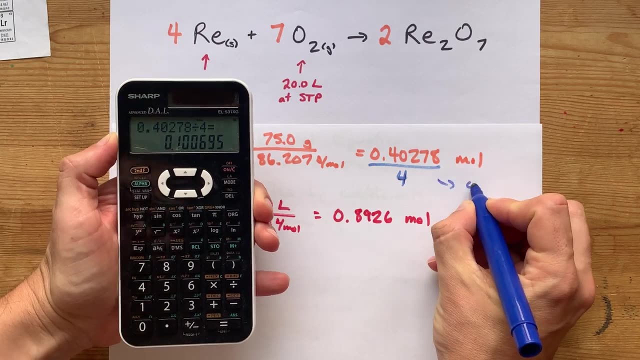 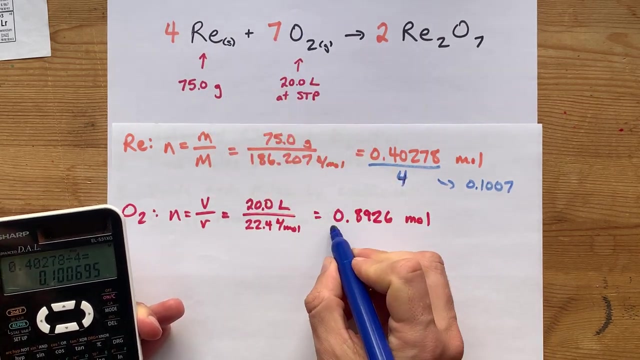 four, Divide by four- I guess I got to do that on my calculator- 0.40278 divided by four, That gives me 0.1007. And oxygen has a coefficient of seven. So I'm going to divide this number by seven. 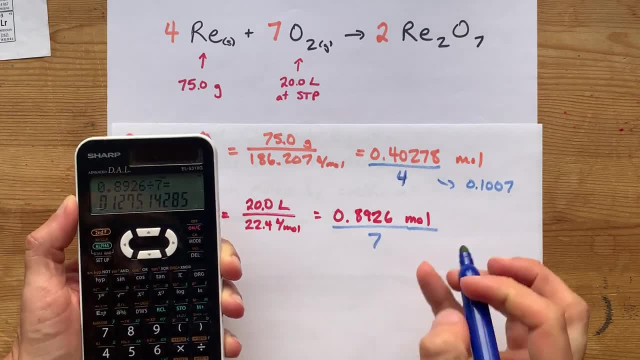 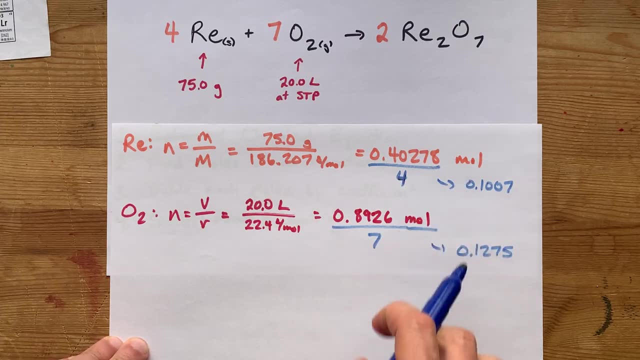 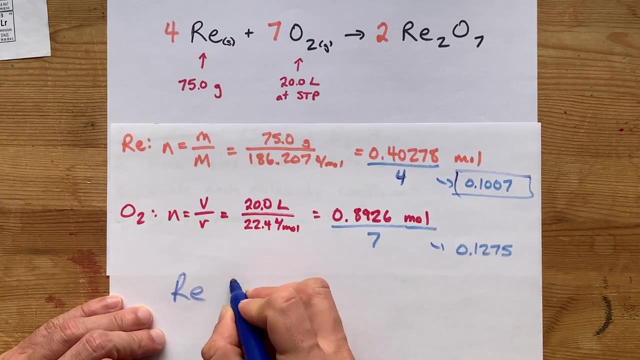 0.8926. divided by seven, That gives me a result of 0.1275.. Now, whichever of those results is smaller corresponds to the limiting reactant. This one's smaller, and therefore RE is the limiting reactant. 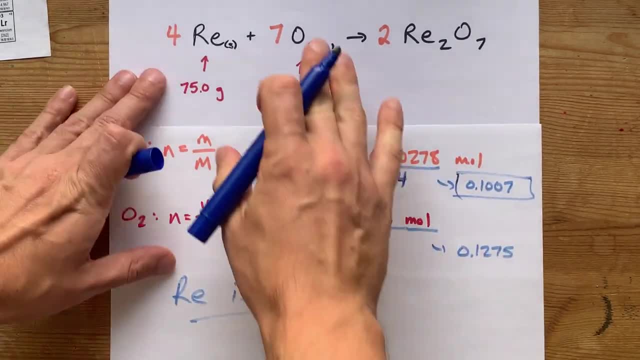 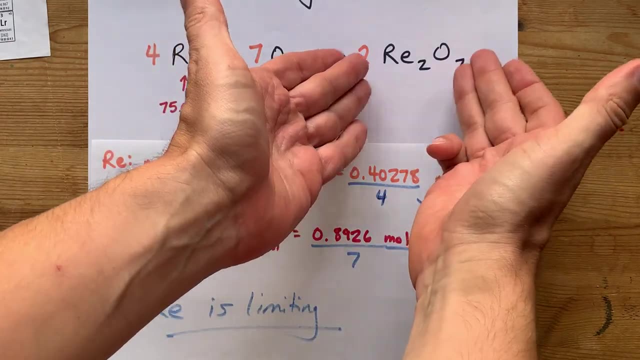 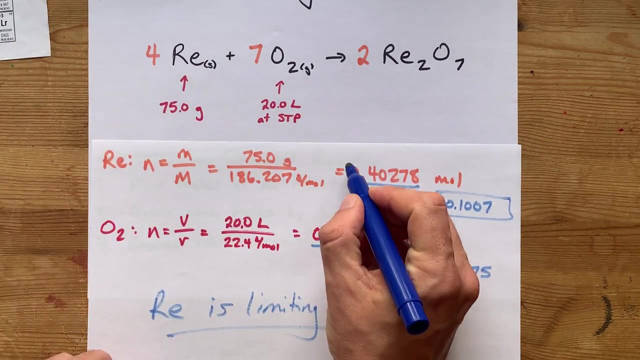 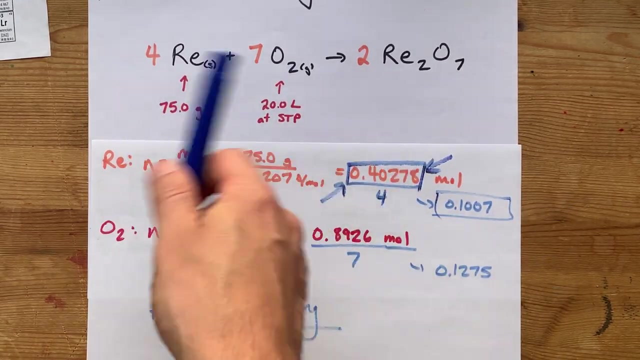 Great, Now that's it. I've answered the question: how to find that limiting reactant. If you're being asked to calculate how much of this is made like the yield of a product, I want you to go all the way back to the number of moles of that limiting reactant and multiply it by a mole.